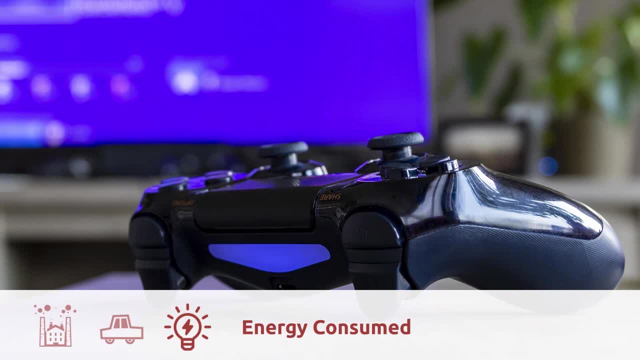 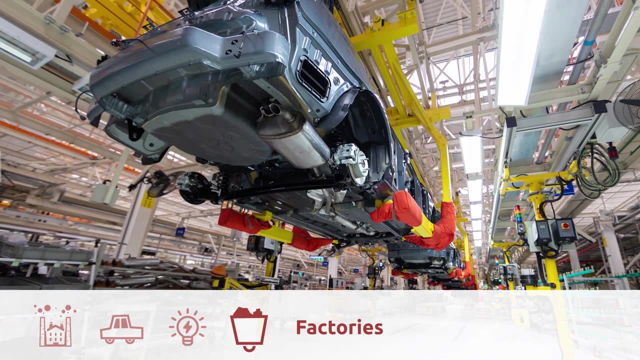 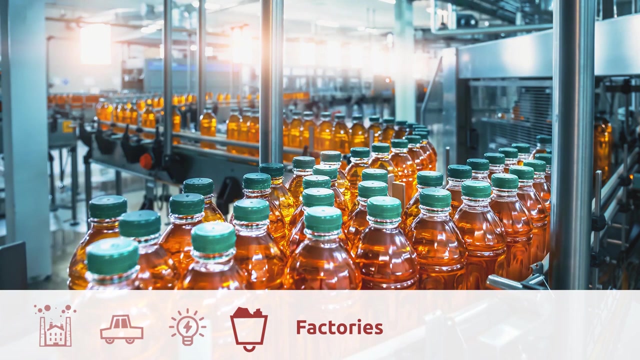 Every time you leave the lights on or any electronic device, you're sending more CO2 to the atmosphere. Factories are another source of CO2 emissions. To produce plastic, for example, We use fossil fuels and we need a large amount of electrical energy to do so. 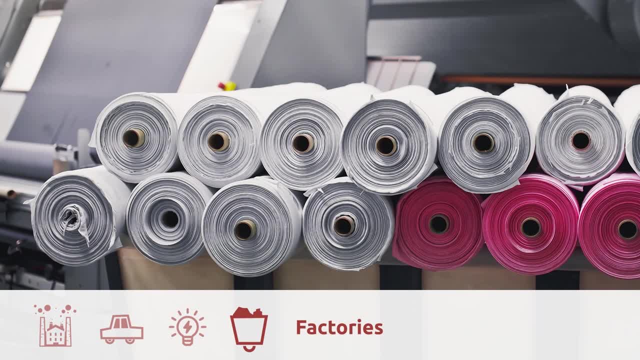 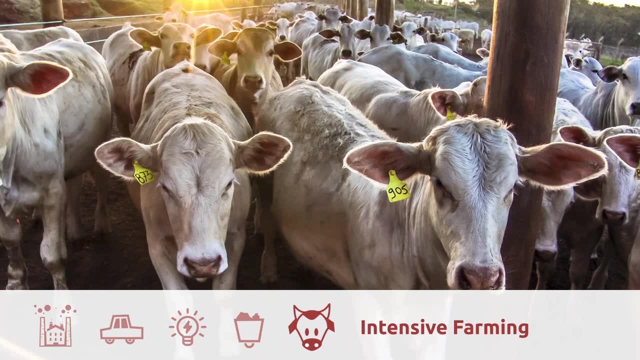 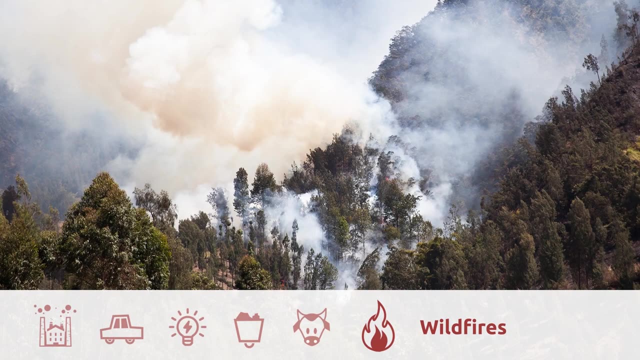 Did you know that the textile industry is highly pollutant? Intensive farming is also responsible for greenhouse effect gas emissions. Wildfires emit large amounts of CO2 in the atmosphere As a consequence of the greenhouse effect. CO2 emissions are generated by the use of fossil fuels. 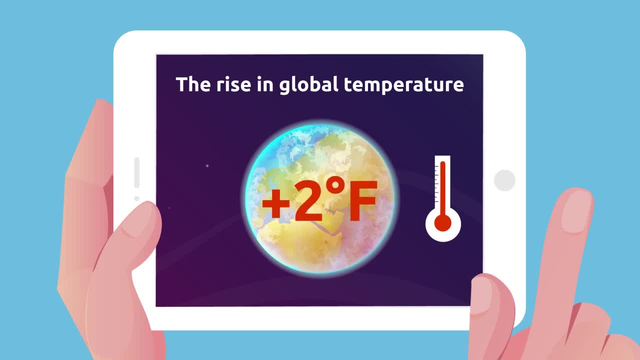 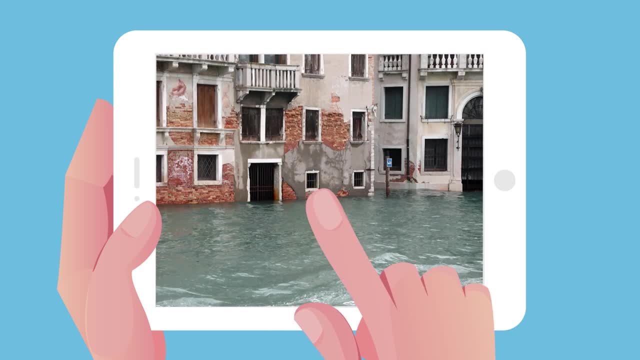 Wildfires emit large amounts of CO2 in the atmosphere As a consequence of the greenhouse effect. CO2 emissions are generated by the use of fossil fuels And the rise in global temperature. The Earth is changing For this reason: water shortage, desertification, the disappearing of lakes. 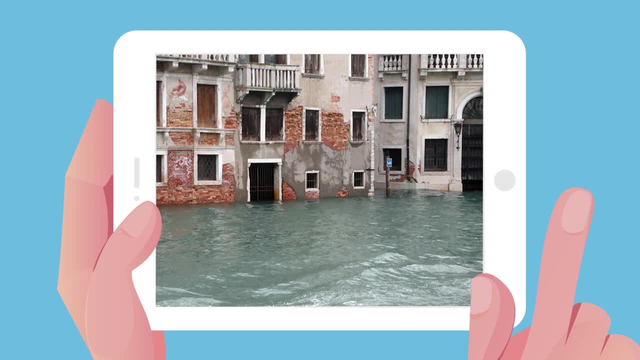 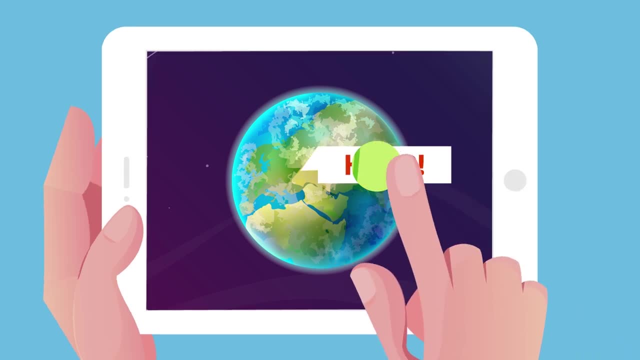 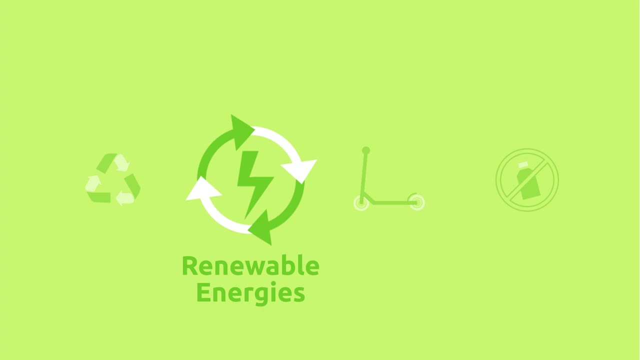 or even sea level rise are becoming more and more common. Worse consequences are predicted in the future if we don't take measures urgently. Currently there are some viable solutions at hand, like recycling using renewable energies, electric transportation or reducing plastic waste. 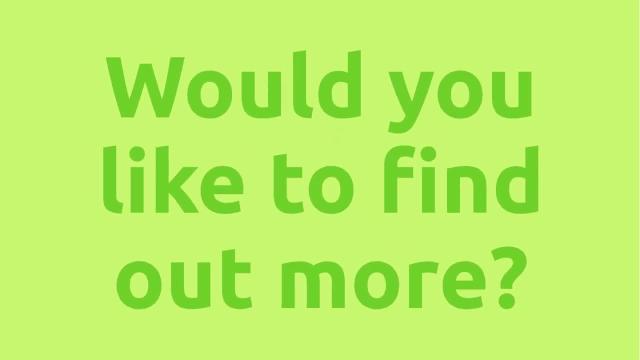 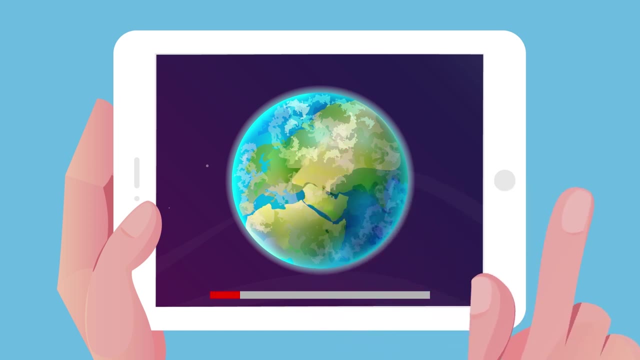 Would you like to find out more? We tell you all about them in our video. Climate Change: We're counting on you. Remember it's in your hands to look after the planet. Want to join us in our mission? Want to join us in our mission? 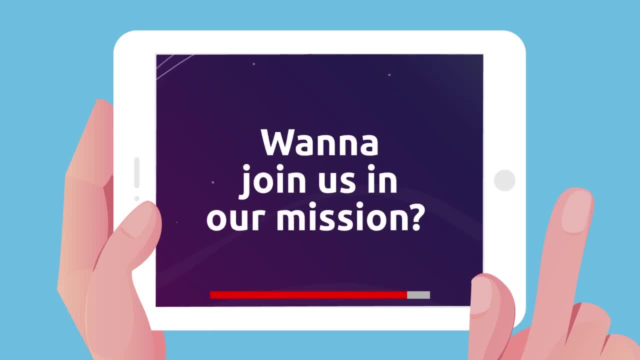 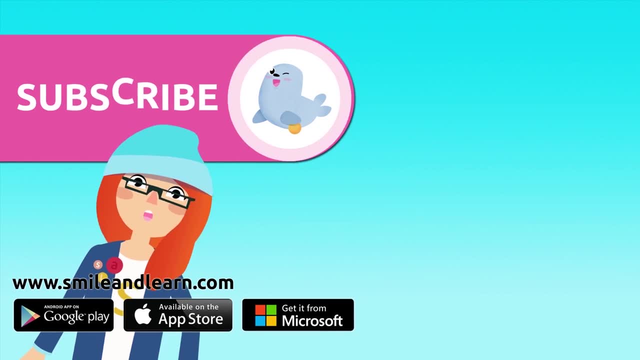 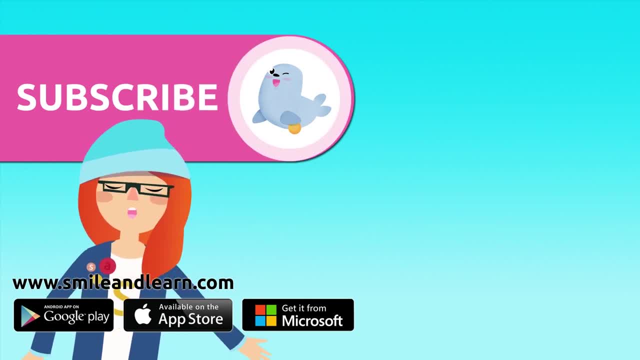 Subscribe by clicking on the seal And if you want to keep watching more videos, click on the boxes. And if you want to keep watching more videos, click on the boxes.